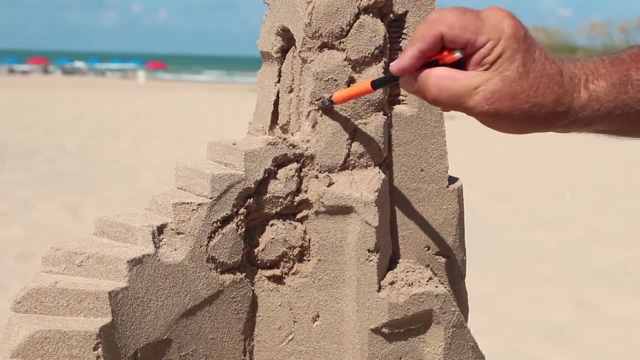 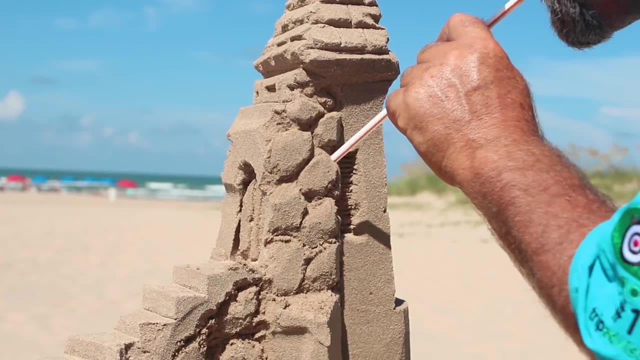 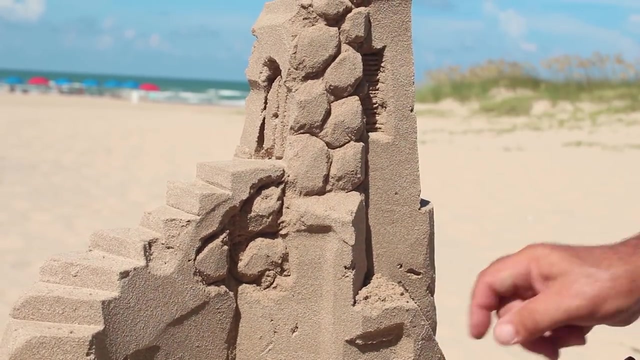 a part of our tower, rip them out And then, once we've done that, of course, what do we use? We're going to use our little paper and we're going to take a pencil and we're going to use our trusty friend. and they're a bit soft. they're a bit hard at the moment, not soft, so we're. 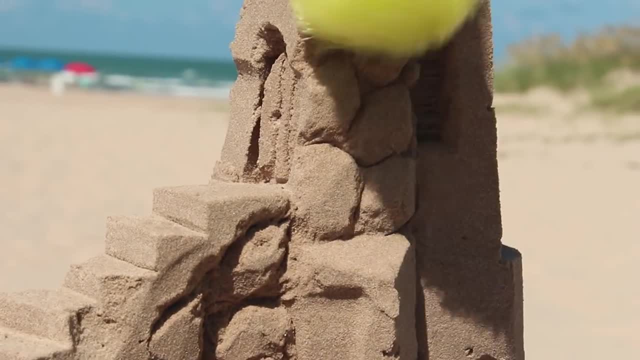 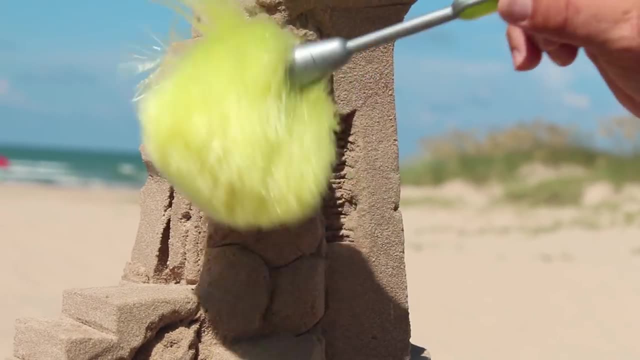 going to make them softer by using the duster very, very slowly. the problem is we don't want to dust everything. you can see this edge. if you touch it with the duster, look what happens to it: it disappears. so the duster is only for when we want blunt, rounded off shapes. we don't use it when we want nice, clean. 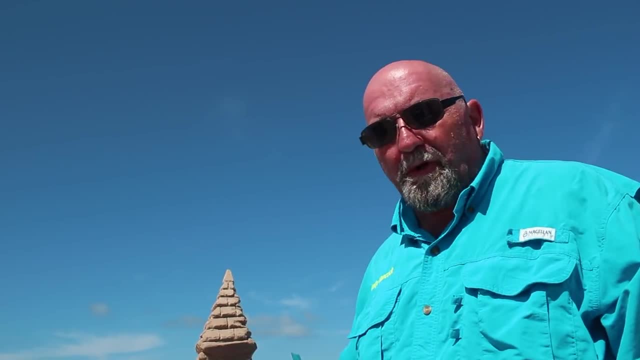 edges once we've carved the top of the stairs as we move towards the bottom of them, we've got to make things a bit more interesting. you could just leave a big slabby old wall with some stairs on it, but we don't do that because we don't do. 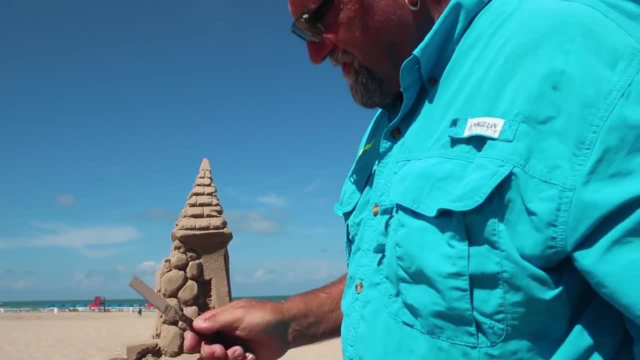 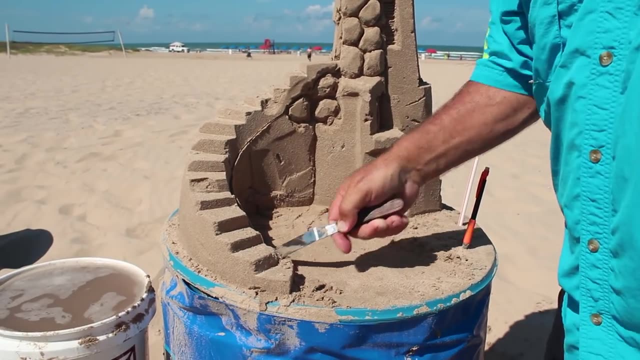 boring says in my shirt. so what we're going to do is introduce a new edge to the underneath of the stair edge like this. so we're going to cut a line right around there and then we're just going to pull all that sander. oh, I've broken. 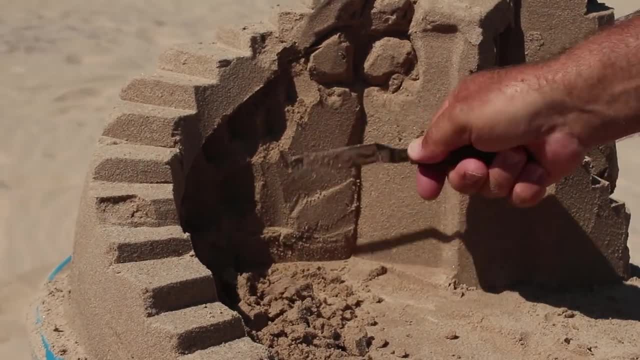 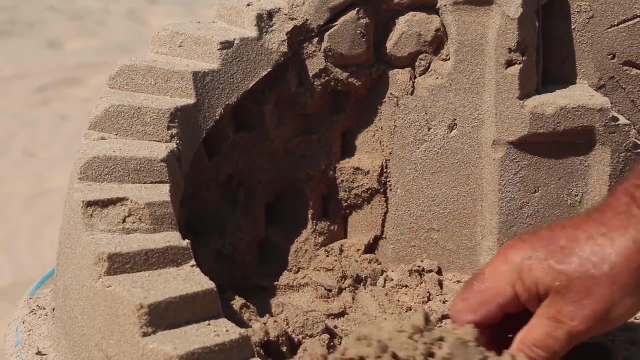 something off. that's terrible. okay, so we're going to take all that sand out of there. but even better than that, we can actually introduce a whole new element to our stairs by pulling that away and you can see. you've got rocks under there. now that's fantastic. 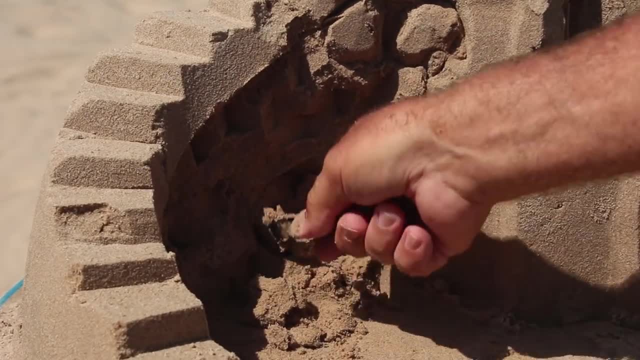 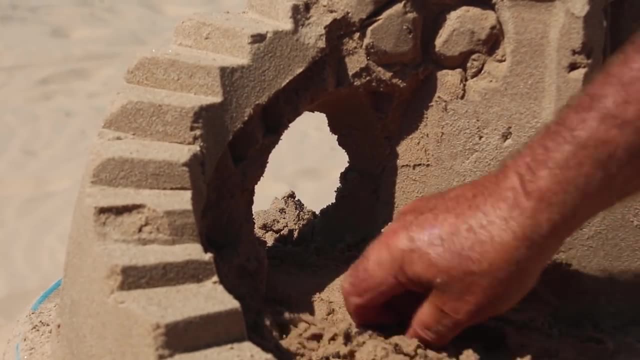 yeah, that's okay, but it's a bit boring. I'll tell you what. why don't we just take some of those rocks out? all right, let's just take the rocks out all together and then take the sand away and just make a whole new arch under our stairs. 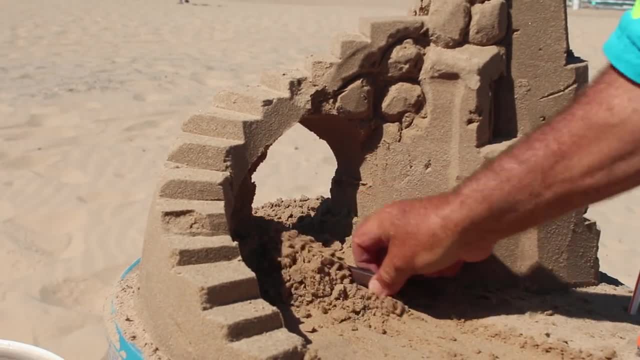 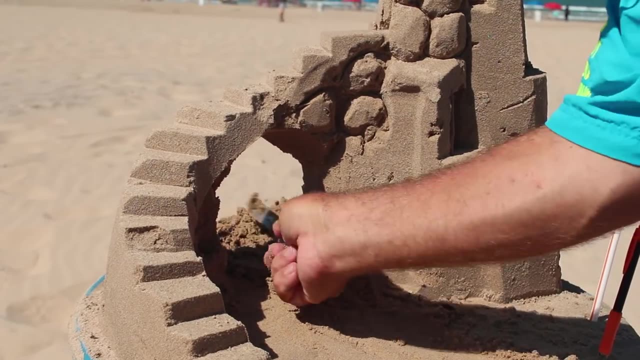 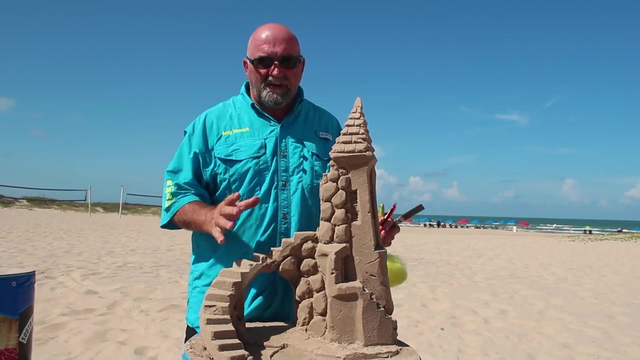 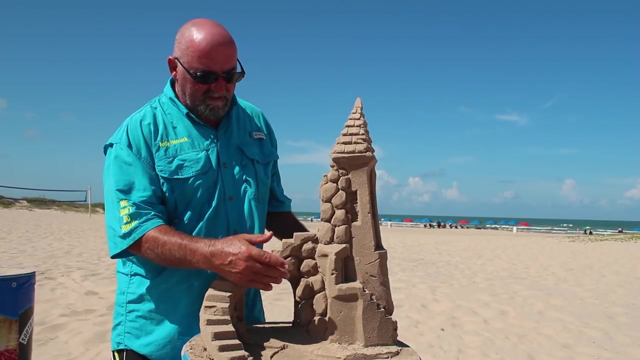 you can see what we're able to create using just our basic toolkit. we can. we can do overlaps, shingles, rocks, bricks, door, stairs, arches, and introduced great contrast. you can see the shadows across the whole sculpture, which actuallyовать you a great contrast. you can see the shadows across the whole sculpture, which 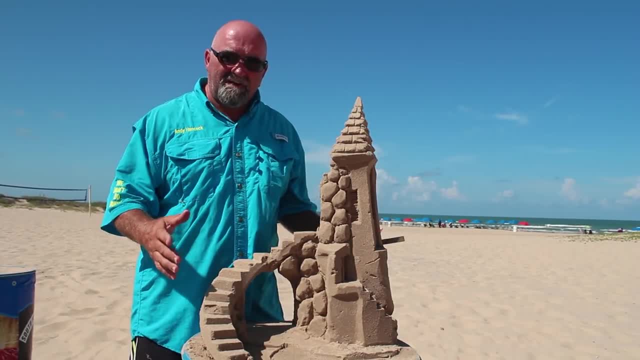 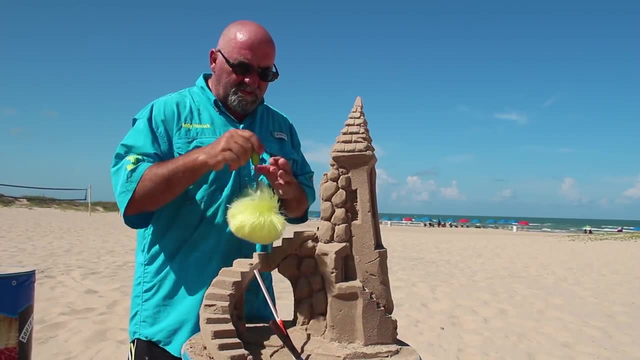 actually lift it to another level. shadow and light and dark is very, very important. we did all this just using our basic toolkit, which is the spatula, the pencil, the straw and, of course, the duster. so it's. this is just so simple. anybody could do it. I'm Andy Hancock. this is South Padre Island, the sand.